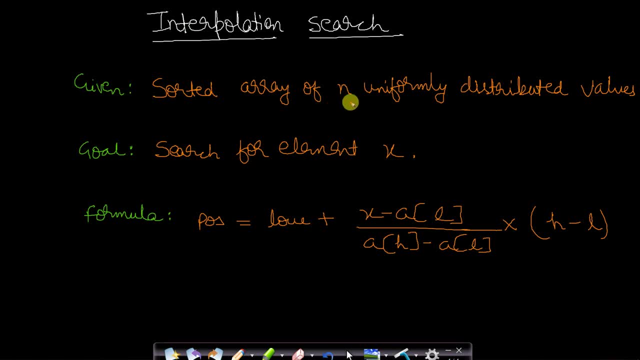 started. We are given a sorted array of n uniformly distributed values. So there are two conditions in order to apply this interpolation search: The given array should be sorted and the elements of the array should be uniformly distributed. What does this uniformly distributed means? 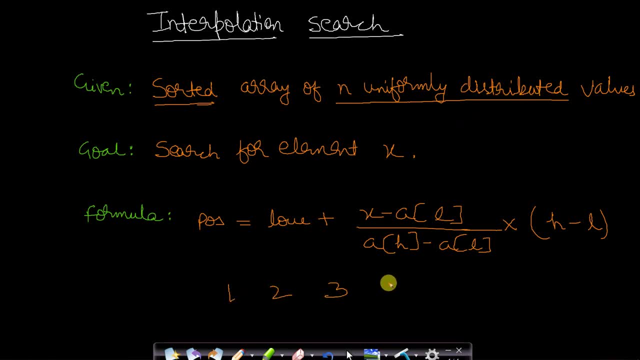 Uniformly distributed means that the gap between the elements should be similar. So let us say we have an array of size 5, then you can see that this is a uniformly distributed array because the gap between these adjacent elements are almost same. Here it is exactly same. 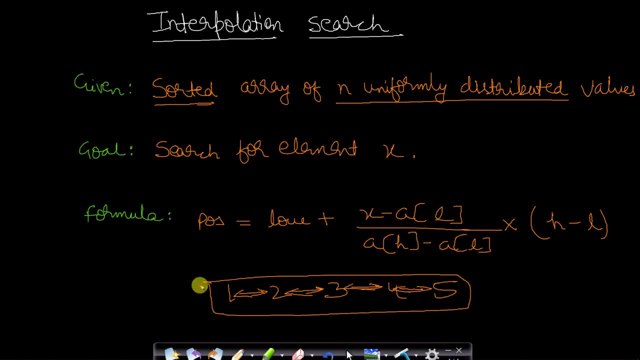 Our goal is to search for element x and how to calculate which index to search for. These are the indexes, The indexes of the array. Now how do we calculate which index to search first? This is calculated by using this formula. The position will get the index where we should look first. What is this? 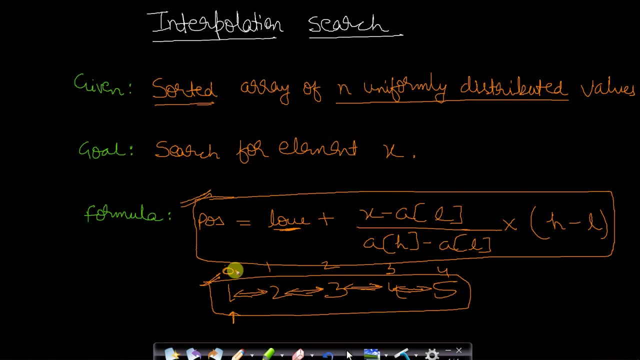 low. This low will be the value of this index. That means here it will be 0.. x is the element to be searched for. a at low is equals to 1 here. a at high minus a at low. a at high is 5 here and. 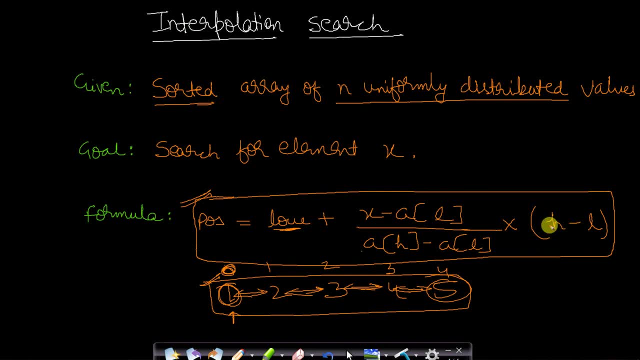 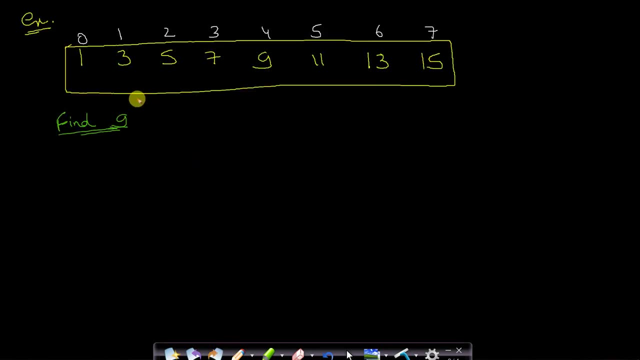 that will be multiplied with high minus low. High index is 4 and low index is 0.. So let us look at how interpolation search works by taking an example. I have already made an array of 8 elements. You can see that they are exactly uniformly distributed. The gap between each. 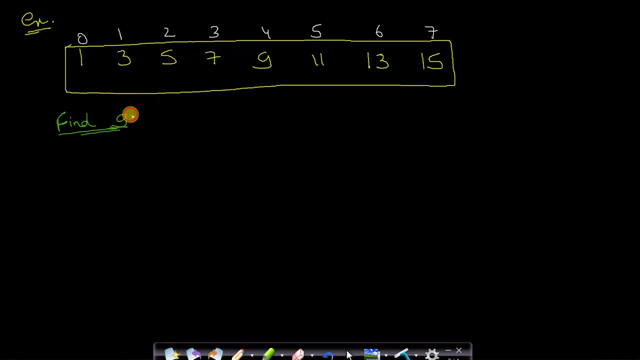 element is equals to 2 and we want to find, let us say, 9.. So what will be the index of 9? and let us say: in how many steps can we find it Here you can see that in the first step of this process, we have 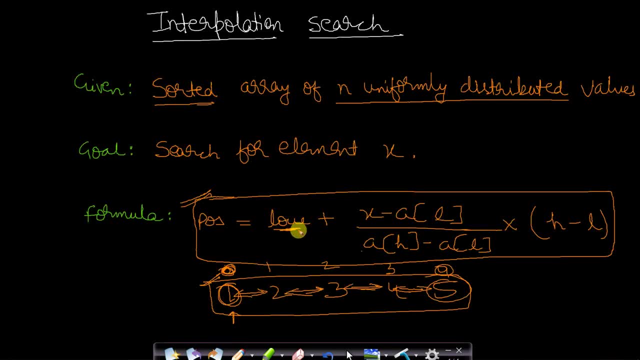 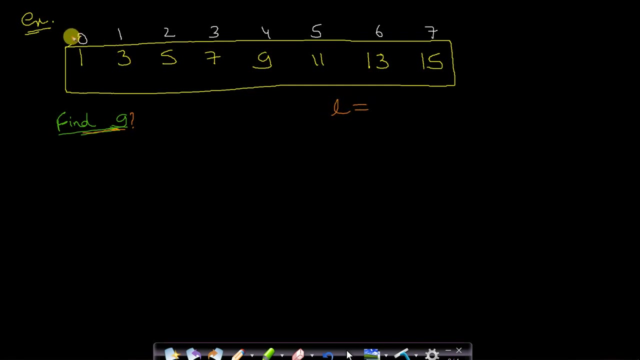 the formula we were required to find this: low, a at low, a at high. this low will be equals to l, actually a at low, a at high and high minus low. these all things should be found out first. so here, low will be equals to the index of the low part, which will be equals to zero, high will. 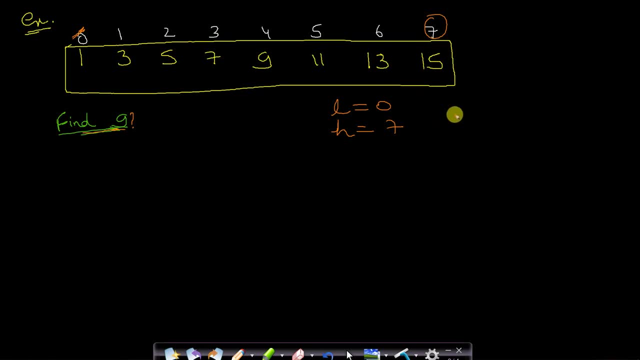 be equals to seven, because it is the index of the high part. now, a at low will be equals to a at zero, which is one. a at high will be equals to a at seven, which is equals to 15. okay, now let us find the position where to look for in order to find nine. so what was our formula? it was low, low plus. 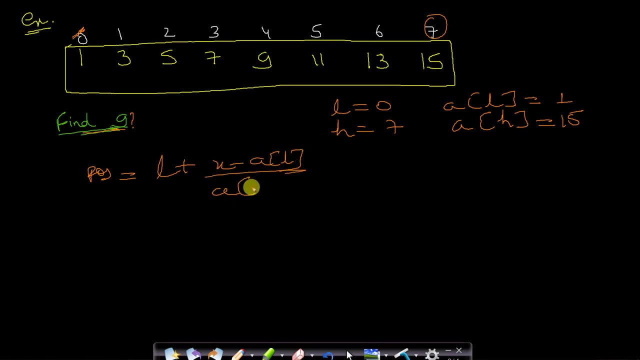 x minus a at low, by a at high minus a at low, into high minus low. so this was our formula. so what is low? low is zero, low index is zero x. the element to be found is nine: a at low equals to one and a at high is 15 and a at low. 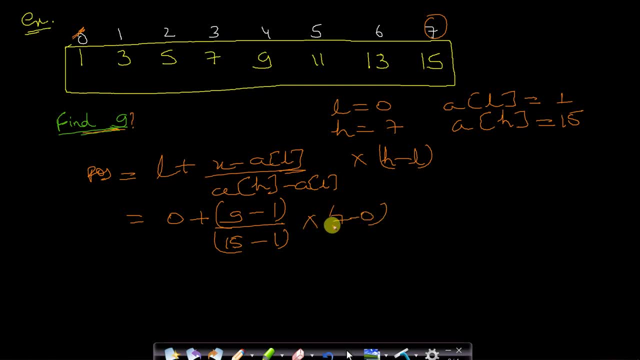 equals to one, and high minus low will be seven minus zero. what will this yield? it will give us zero plus eight by fourteen into seven, and this will give us four. so we should look at the fourth index in order to find nine. so, on looking at the fourth index, you can see that it matches the 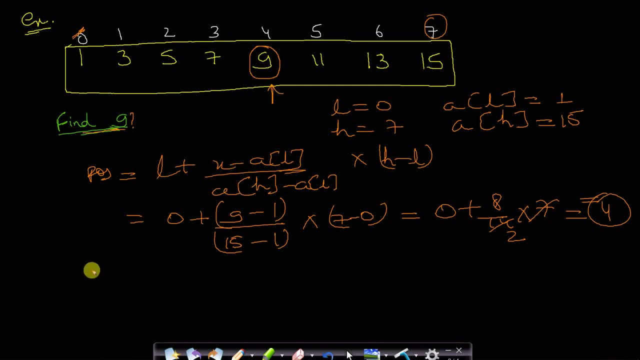 element to be found, which is nine. so you can say that we have found this nine in just one step. we found this nine in just a single step. what would have happened if we would have used binary search? you know that binary search takes log n time, so how many steps would have been performed here if? 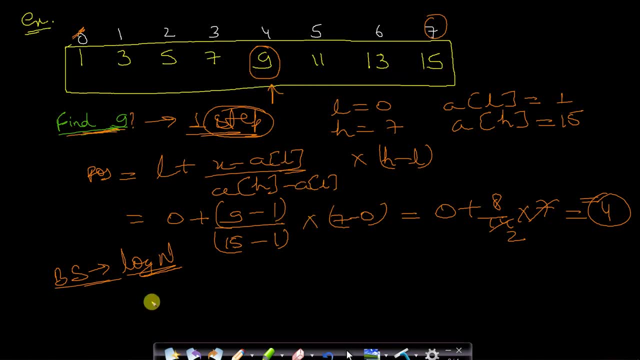 you take this entire array, then the middle element will be considered, and what will be the middle element? the middle element will be seven by two, a, this low plus high by 2. so low is 0 and high is 7. so 0 plus 7 by 2 will be equals to 3. 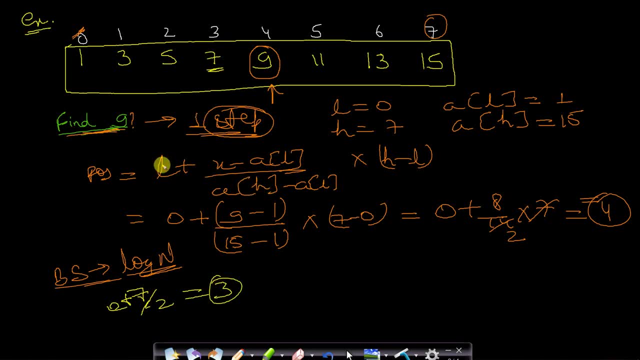 so first this 7 would have been matched. now 7 is not equals to 9 and this 9 is greater than 7. so this array would have been divided into two parts. and now this 4 would have been low, this 7 would have been high and the middle element would have been 7 plus 4 by 2, and that would 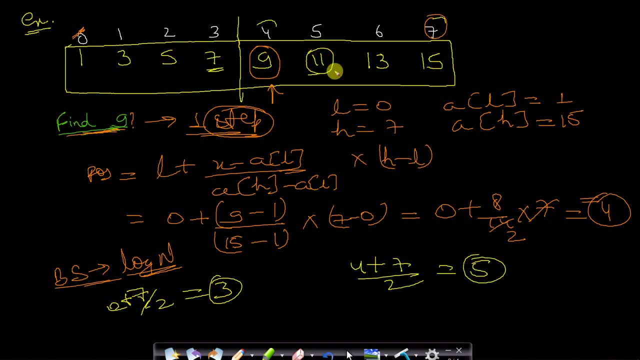 have given 5, now we would have compared this 11 with 9, and this also would not have given us the result. and so, since this 11 is greater than 9, so we would have divided this entire array into two parts, and now only this part would have been left, and now we will find 9. so the number of steps in 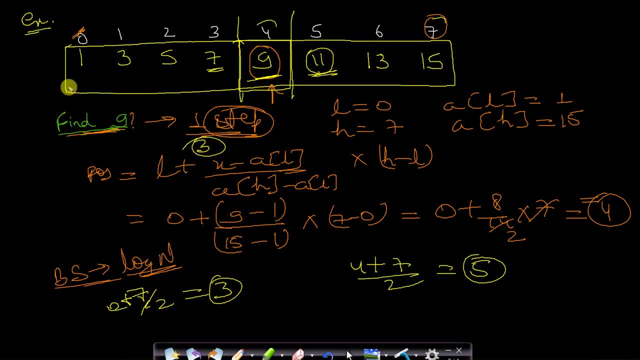 this case would have been equals to 3. so you can see that if the array is sorted and it is uniformly distributed- that means the gap between the array elements are almost similar- then interpolation search is the best searching algorithm here to apply. In this case it takes only one step to find 9, while binary search would have taken. 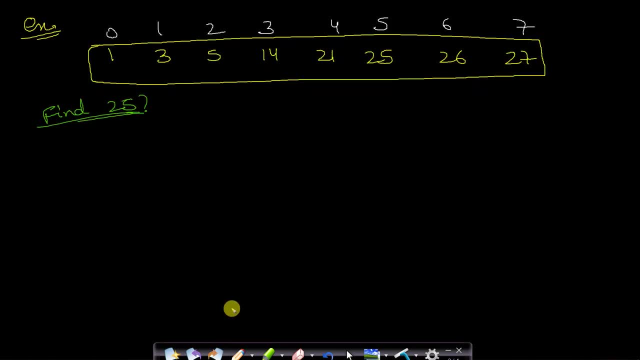 three steps. Let us look at another example in which the array is not so uniform as we had seen in the previous example. So you can see that the difference between these two elements is 2. while the difference between these two elements is larger, It is equals to 9.. So this array's 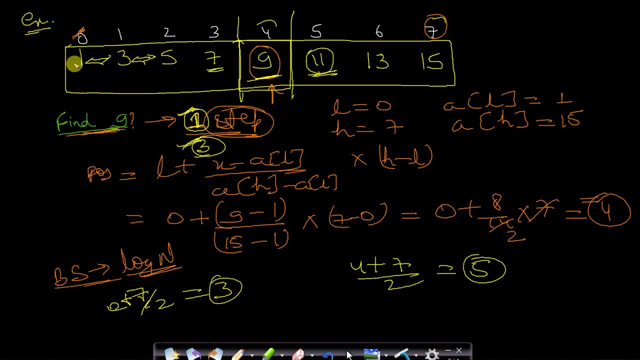 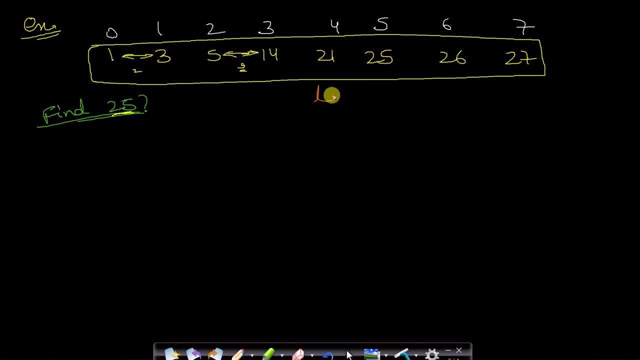 uniformity is less as compared to the previous array, where the uniformity was exactly similar. In this array, let us find 25.. Now we need some values. We need low. Low is equals to 0.. High equals to 7.. A at low will be equals to 1.. A at high will be equals to 27.. This is the initial. 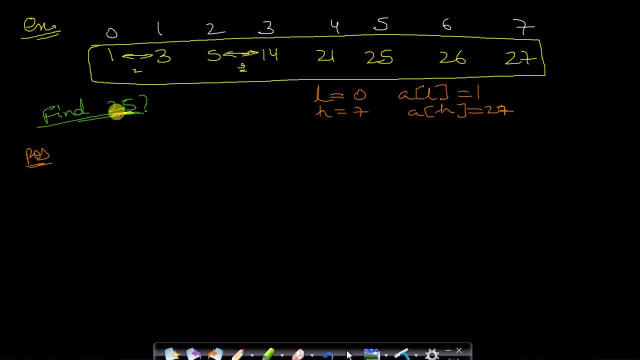 assignment. Now we want to find the position where to look for in order to find 25.. This will be equals to low plus x. that is 25 minus array at low, which is equals to 1, and then array at high minus array at low. that means 27 minus 1 into high minus low. This will be 7 minus 0.. So what will be the value? 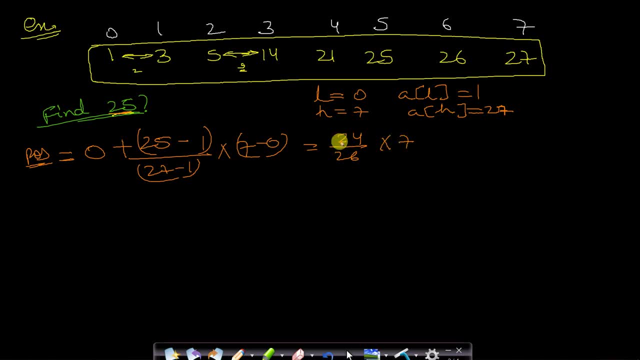 here It will be 24 by 26 into 7, and this will be 12.. This will be 13 and this will come out to be 84 by 13, and I think this will be almost equals to 6. okay, because we will be taking the floor value, It will be 6.. Now, what we will do is we will look. 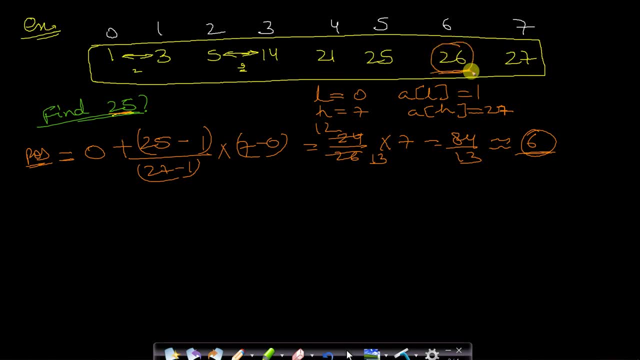 for 25 on the 6th index, but the 6th index is equals to 26.. Now what we will do is we will divide this array into two parts and since this 26 is greater than 25, so we will take the left half. 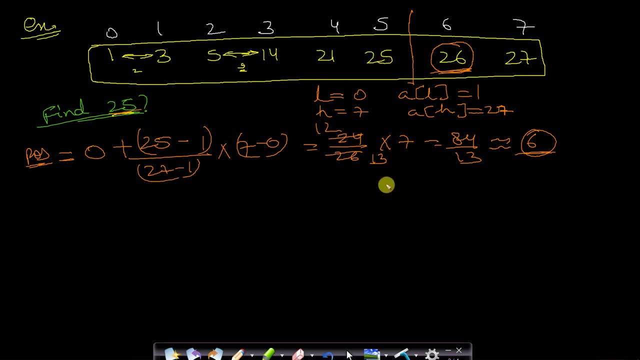 and we will search for 25.. Now we will reassign the values. So what will be the new values? The new value of low will be 0, of high will be equals to 5.. A at low will be 1. A at high will be equals. 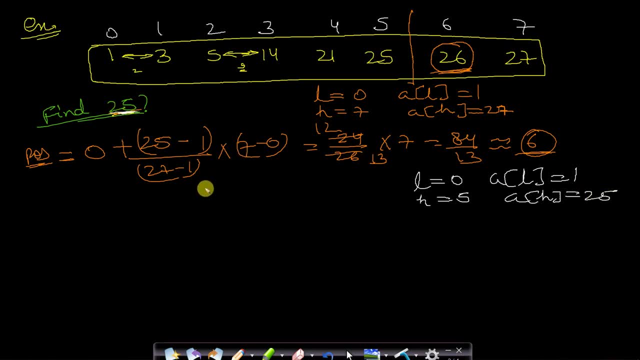 to 25.. Now we want to search for 25.. Now how do we find it? If we write position, then this will be equals to low plus x minus array at low. Array at low is 1. By array at high minus array at low into high minus low. So the high index is 5, low index is 0. 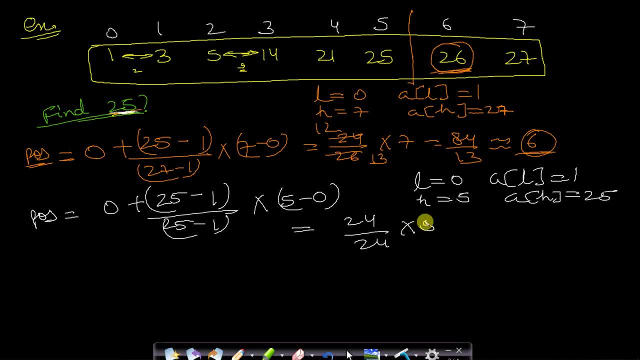 This will yield 24 by 24 into 5 and this will be equals to 5.. So it says that we should look at index 5 in order to find 25, and you can see that we found 25.. So the number of steps which are: 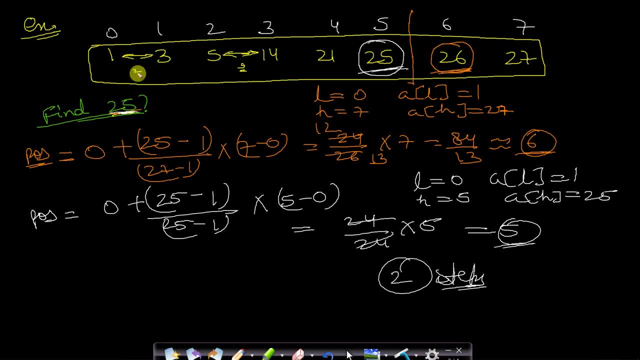 in two steps and why two steps were required? because this array is not exactly uniform. The gaps between the elements are exactly the same. Then we will definitely find, given any element, we will find in just a single step. If we are taking more than one step, then we can say that array is: 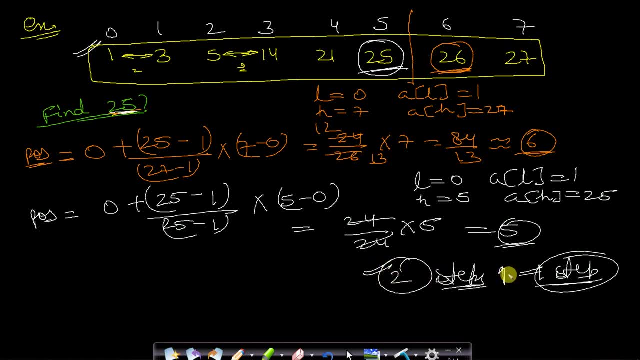 not that uniform, and if the number of steps taken increases, then the uniformity of array can be said to be less, Because if the array is less uniform, then the number of steps will increase. In this case, we found 25 in two steps. What would have happened if we had applied binary search? Let us 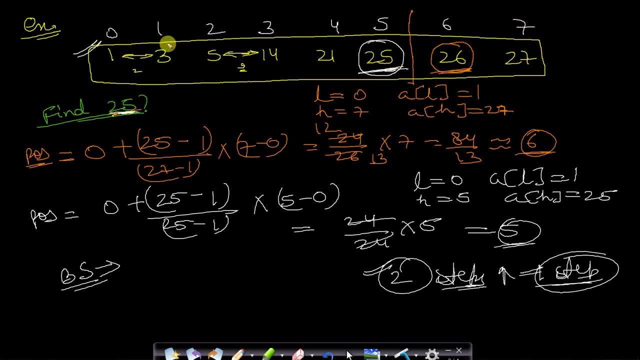 see by applying binary search. The middle element for this first will be 0 plus 7 by 2, which will be 3.. So we will look at this: 14.. 14 is not equals to 25 and 14 is less than 25.. So we will divide this. 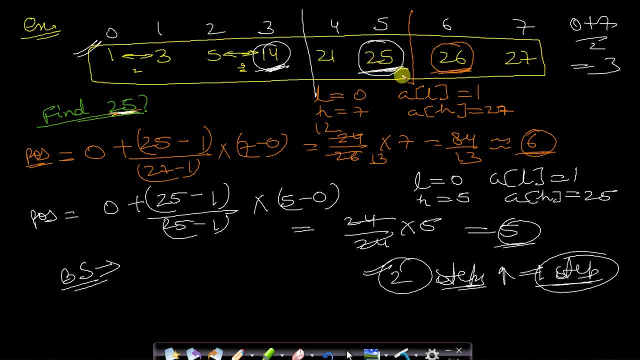 into two parts and we will look for 25 in the right hand side. So now the middle element will be 7 plus 4 by 2, which will be equals to 5.. So we will look at index 5 and at index 5 you can see that we have found the element. So binary search would have.